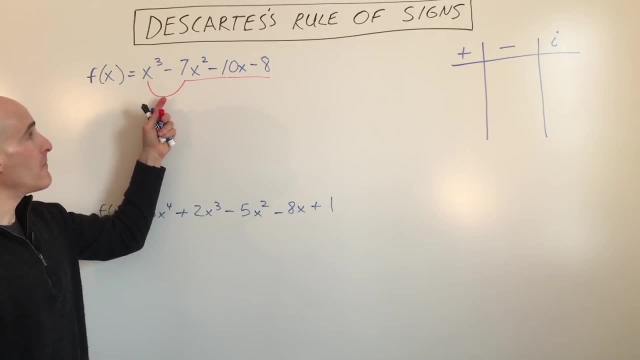 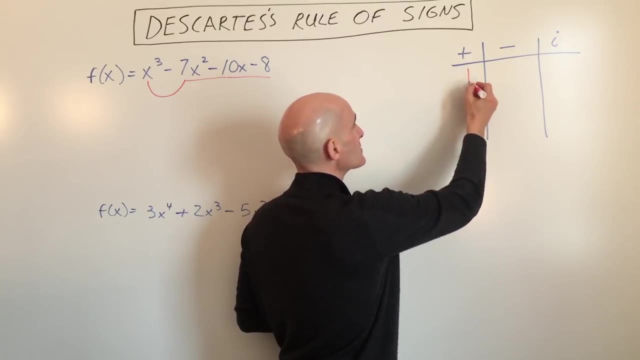 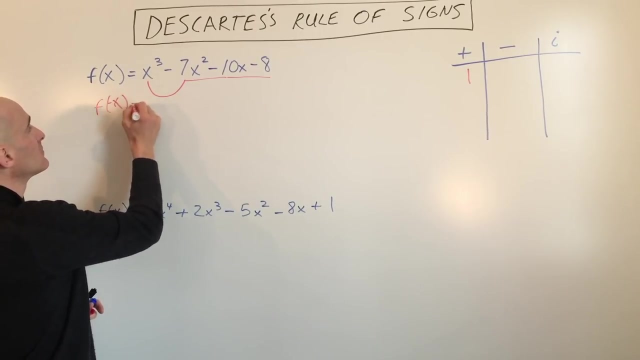 also doesn't change signs. So what that tells us is that we have a maximum of one positive zero. Okay, so that means we're going to have a maximum of one. Now what we're going to do is we're going to substitute in negative x into our function And we're going to analyze. 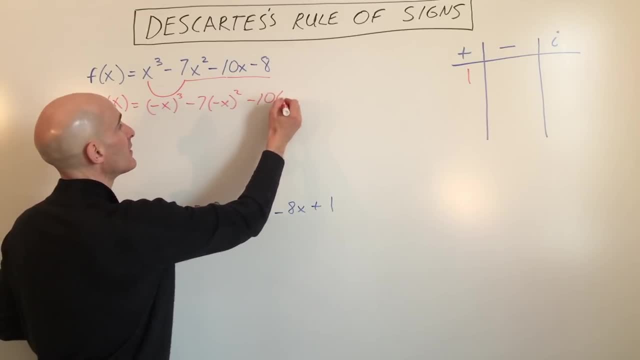 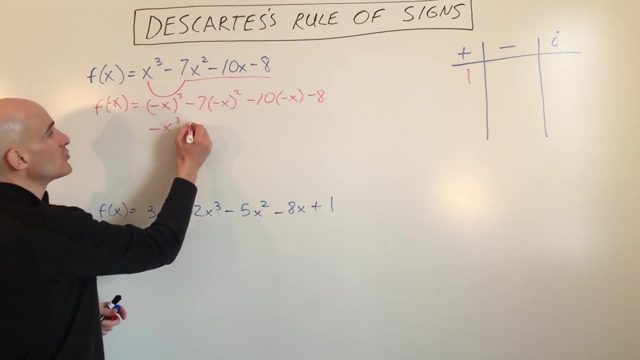 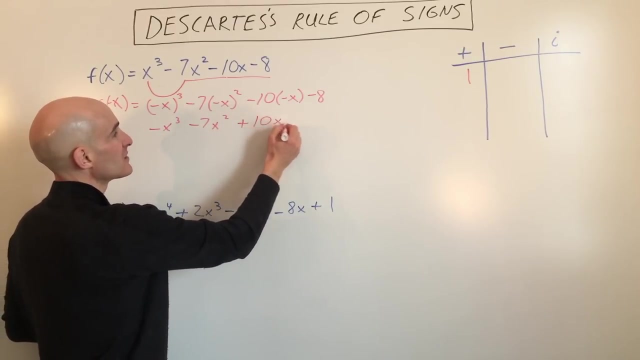 the sign changes after we simplify The function with negative x substituted in place of x. So here we're going to get negative x cubed, negative, 7x squared, because a negative squared is positive. Negative times negative gives you positive 10x minus 8.. Okay, so now let's count the sign changes. We have negative. 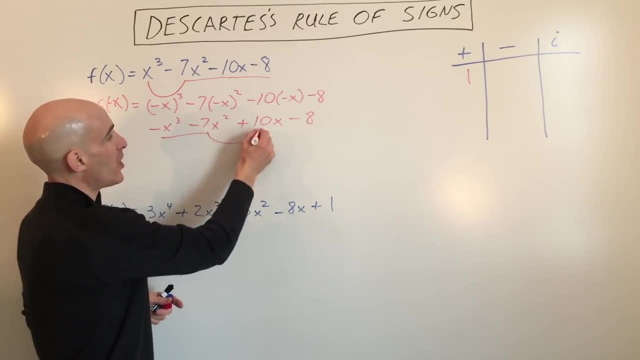 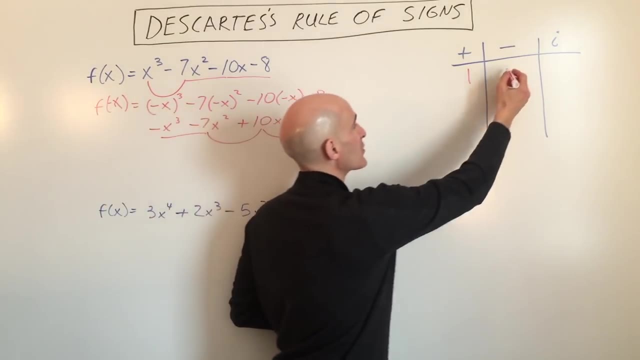 to negative. negative to positive: that's one. Positive to negative: that's two. So that means that we have a maximum of two positive- I'm sorry, two negative. So we have a maximum of two negative zeros. So what that means is on your graph it's going to cross over. 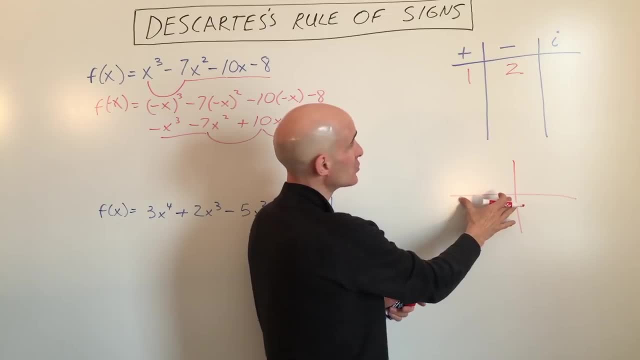 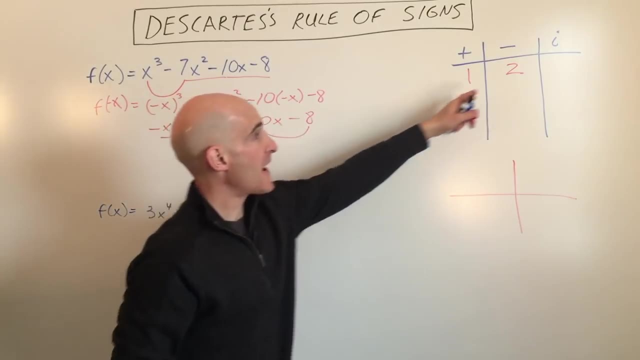 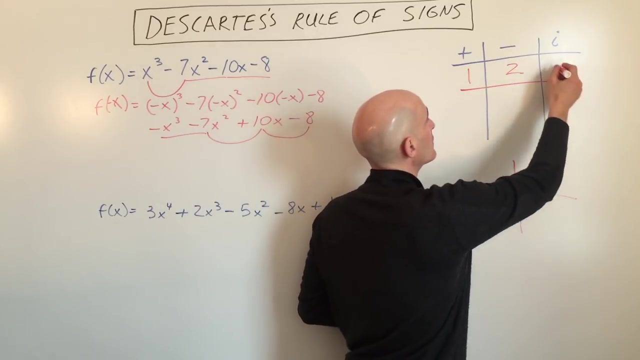 here, in the negative okay range a maximum of twice and in the positive range, a maximum of once. But these are the maximums Okay and what you can see is this is a third degree. So as we add across this row here, these add up to three, But when you have real coefficients, 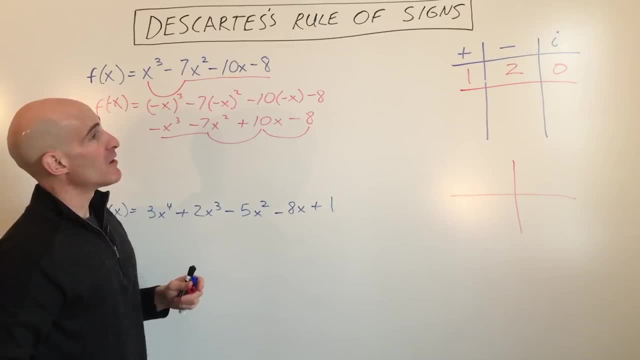 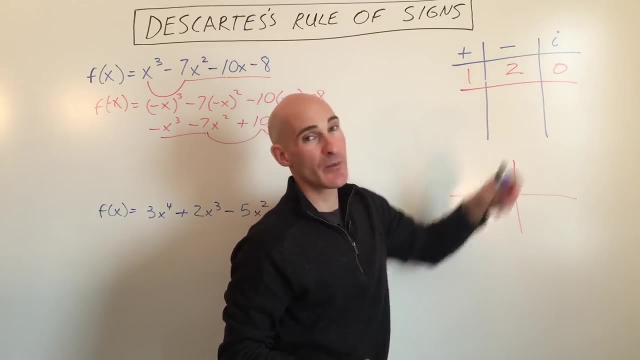 these numbers here in front of the video, these numbers here in front of the video, the variables. if these are all real, then if you have any complex roots, complex zeros, imaginary solutions, they're going to come in what they call conjugate pairs. So for 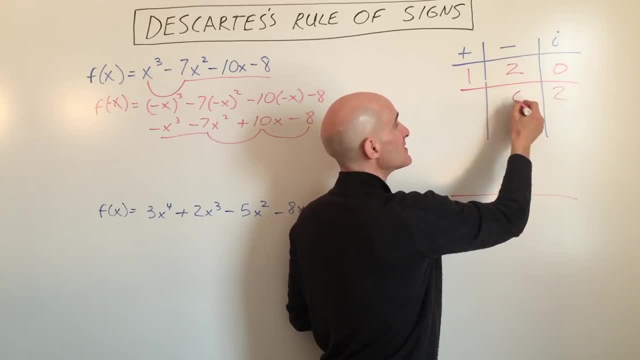 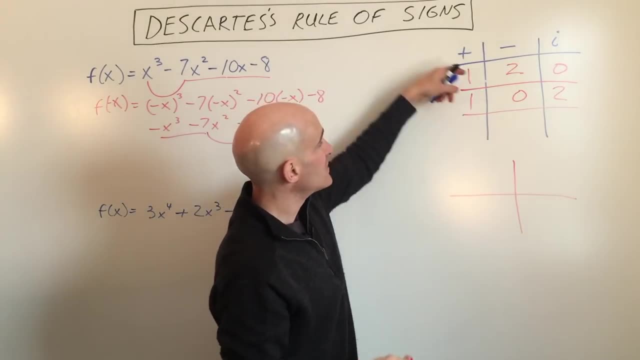 example, you could have two imaginary zero negative and one positive. So when you work with Descartes' Rule of Sines, you take these maximum values and you can decrease them by two, four, six, eight, by groups of numbers. Okay, so that's two, four, six, eight by. 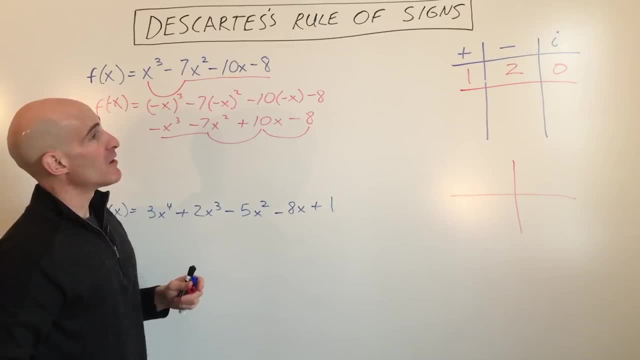 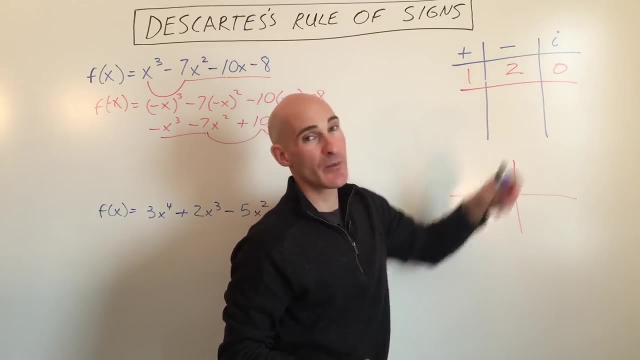 these numbers here in front of the video, these numbers here in front of the video, the variables. if these are all real, then if you have any complex roots, complex zeros, imaginary solutions, they're going to come in what they call conjugate pairs. So for 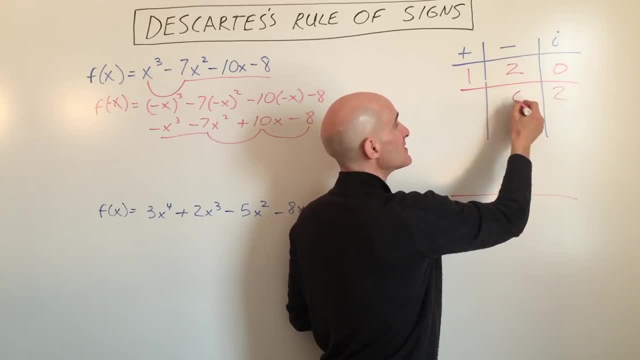 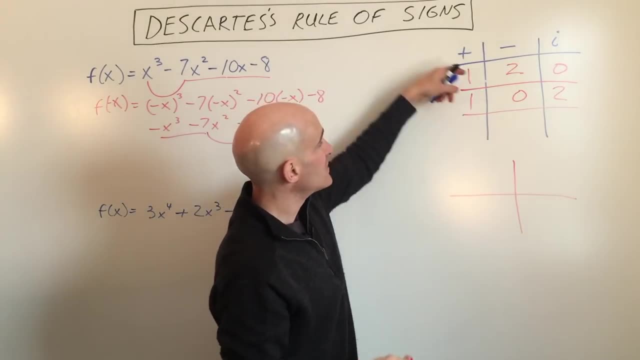 example, you could have two imaginary zero negative and one positive. So when you work with Descartes' Rule of Sines, you take these maximum values and you can decrease them by two, four, six, eight, by groups of numbers. Okay, so that's two, four, six, eight by. 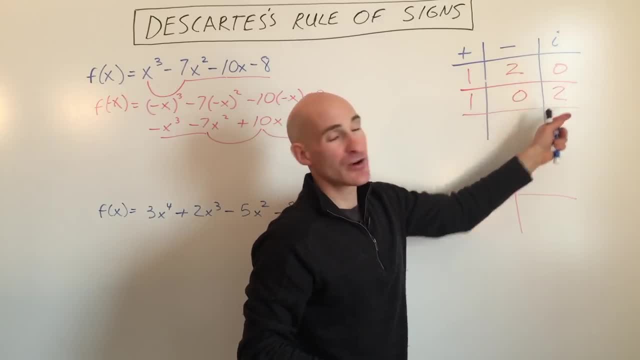 groups of numbers: Okay, so that's two, four, six, eight. by groups of numbers: Okay, so that's two, four, six, eight. by groups of numbers: Okay, so the imaginary ones are going to increase by groups of two. The imaginary ones are going to increase by groups of two. 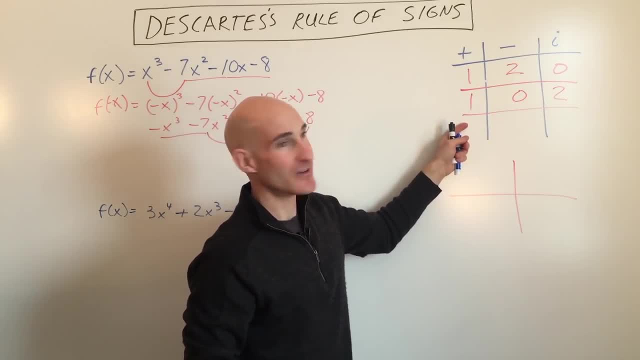 So this one I wasn't able to subtract two from because that would put me into the negative number of positive zeros. you can't have a negative number of positive zeros And you can't take away an odd number, only an even amount. So take two, four, six away, and these 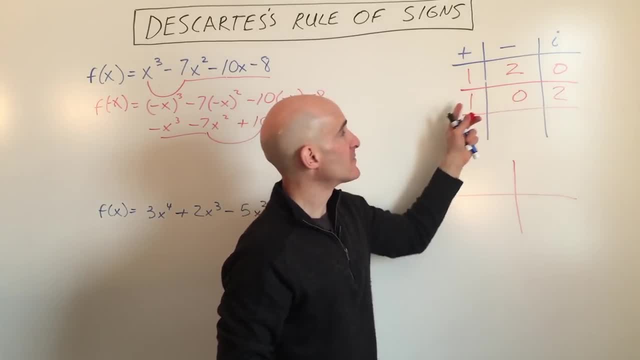 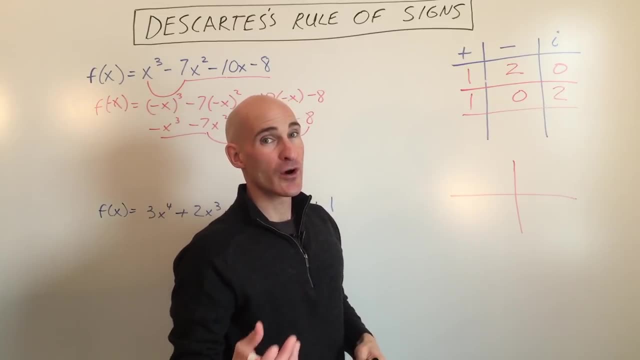 are going to increase by two, four, six. So these are our only possibilities for the zeros for this function. So if I was doing synthetic division, I would be taking the negative number out of the division and I was looking for a possible zero. I would start by looking for a positive one first. 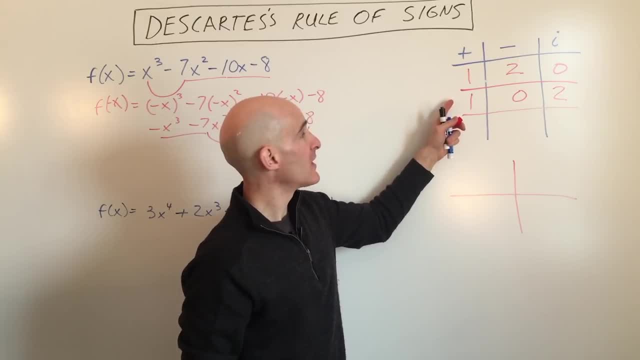 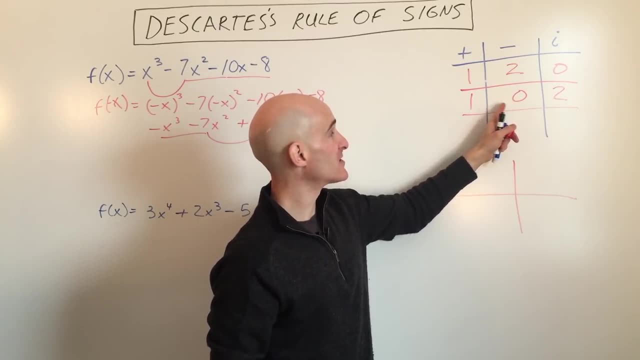 because I know that there's at least one positive one. If it's this scenario here, I might be looking for a while for a negative zero and not actually be able to find one, because there's just going to be two imaginary and one positive. So what Descartes' rule of science does is it helps. 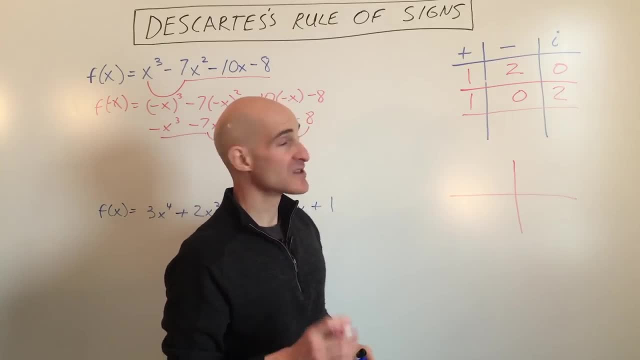 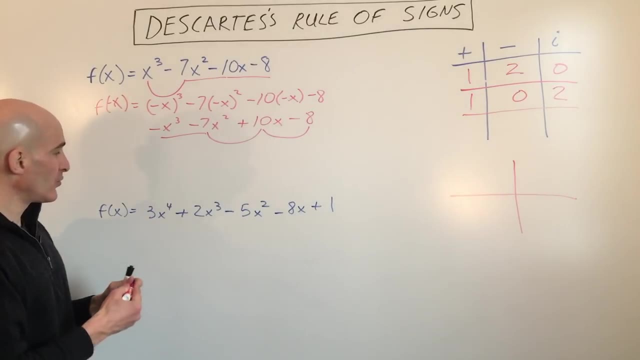 you narrow down your choices when you're doing the synthetic division to find possible rational roots. Okay, so let's take a look at another example. This example here. let's count the number of sign changes, So we have positive to positive, positive to negative. that's one. 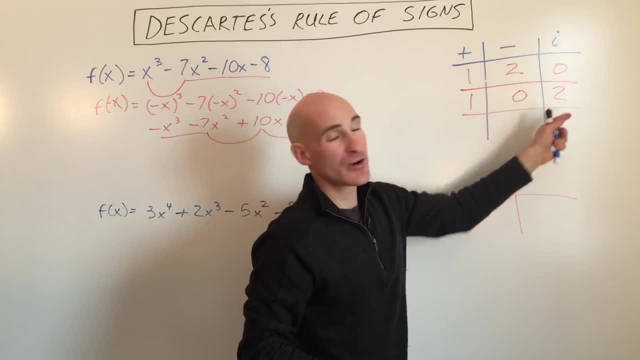 groups of numbers. Okay, so that's two, four, six, eight. by groups of numbers. Okay, so these numbers are going to increase by groups of two. The imaginary ones are going to increase by groups of two. So this one I wasn't able to subtract two from, because that would put 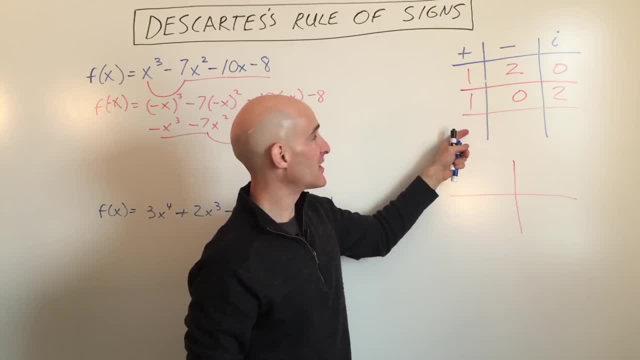 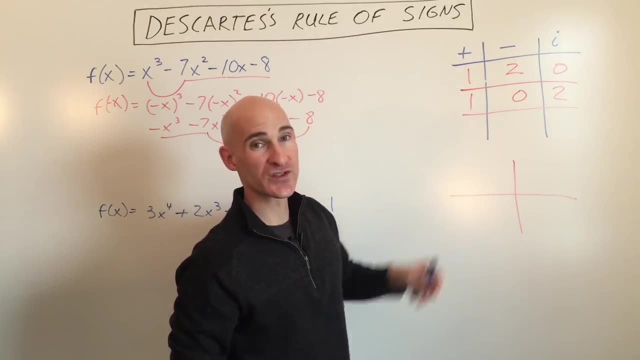 me into the negative number of positive zeros. You can't have a negative number of positive zeros And you can't take away an odd number, only an even amount. So take two, four, six away and these are going to increase by two, four, six. So these are our only possibilities. 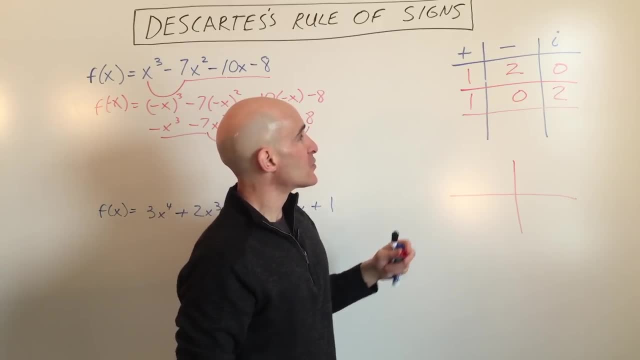 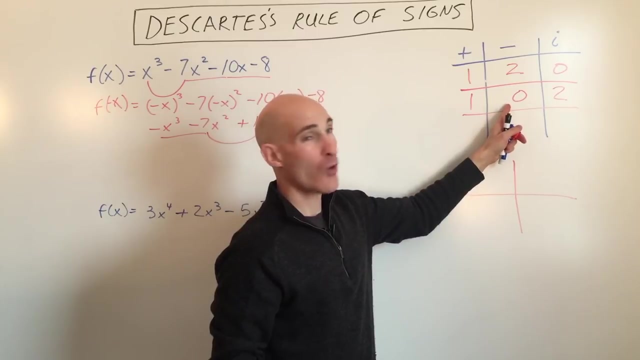 okay for the zeros for this function. So if I was doing synthetic division and you division and I was looking for a possible zero, I would start by looking for a positive one first, because I know that there's at least one positive one. if it's this scenario here, I might be looking for a while for a negative zero. 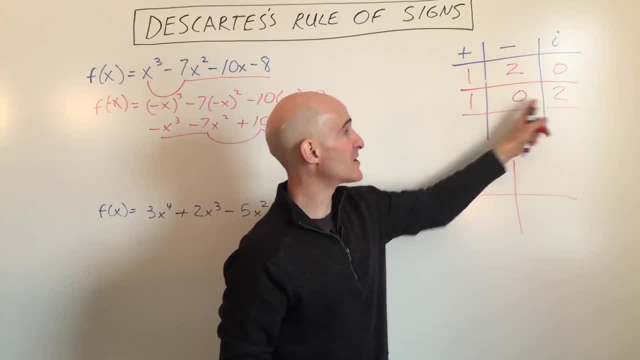 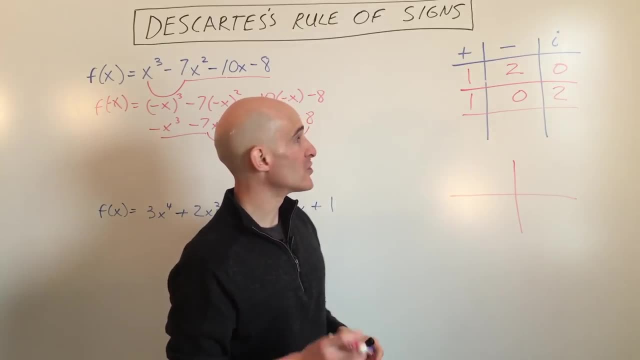 and not actually be able to find one, because there's just going to be two imaginary and one positive. so what Descartes rule of science does? it helps you narrow down your choices when you're doing the synthetic division to find possible rational roots. okay, so let's take a look at another example. this: 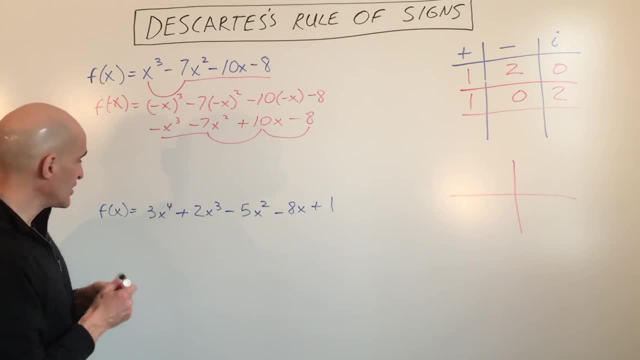 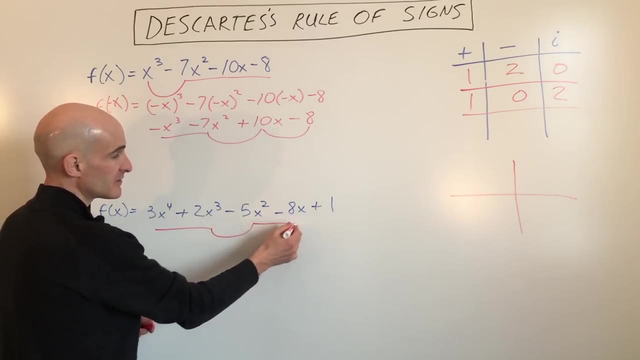 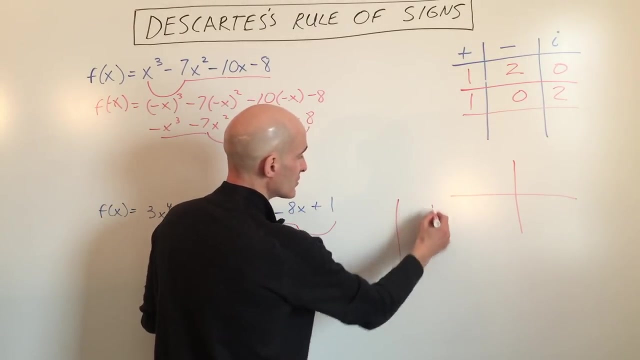 example here. let's count the number of sign changes. so we have positive to positive, positive and negative, that's one. negative to negative doesn't change. negative to positive, that's another one. so what we have here is let's make another one of our charts- positive, negative, imaginary we're going to have a 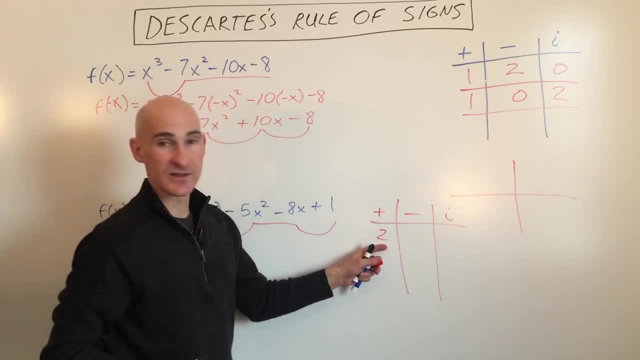 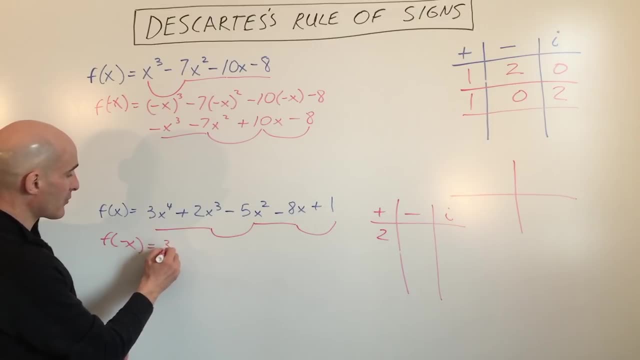 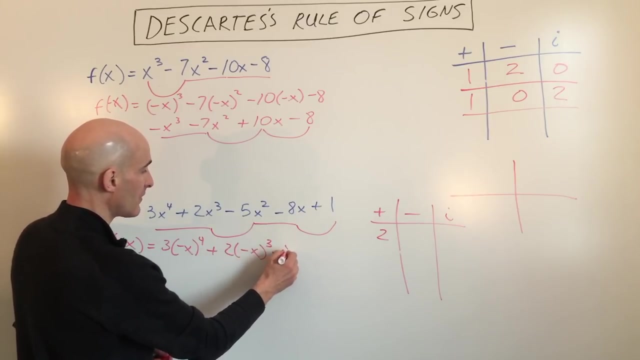 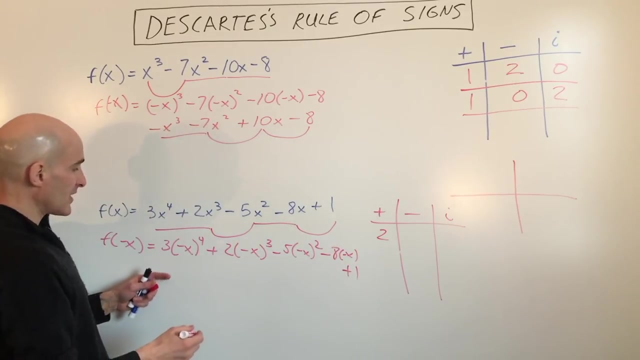 maximum of two positive zeros. if we substitute in negative x, we're going to get okay. so f of negative x, we're going to get three times negative x to the fourth, plus two times negative x, cubed, minus five times negative x, squared, minus eight times negative x plus one. okay. so here, if we simplify, we get positive three x to the. 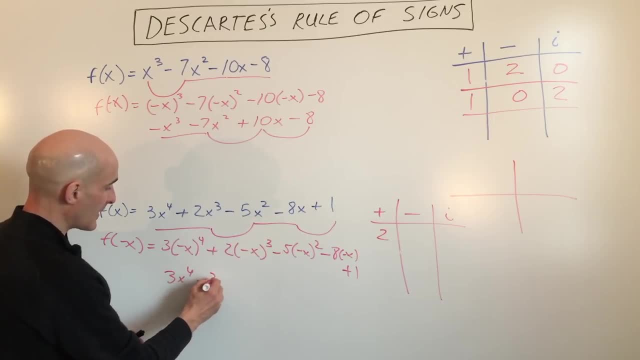 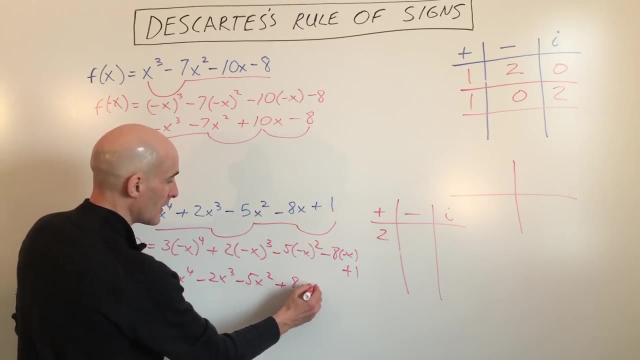 fourth, because a negative to an even power is positive. we're going to get minus two x cubed. we're going to get minus five x squared. we're going to get positive eight x and plus one. so now let's count the number of sign changes. we have positive. 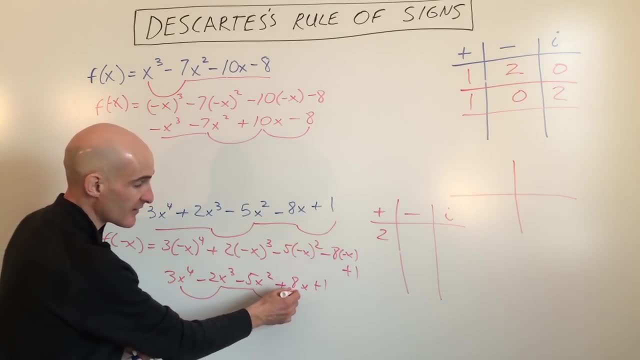 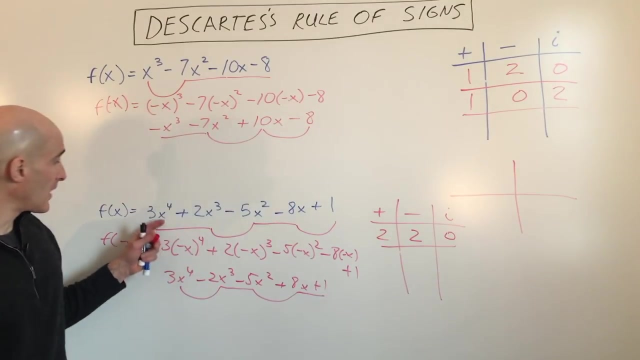 negative- that's one negative. negative that doesn't change. negative. positive: that's two positive, positive that doesn't change. so we have a maximum of two negative zeros. okay, so these are the maximum, and if we add across two plus two plus zero gives us four, and the maximum number of zeros you can have is whatever. 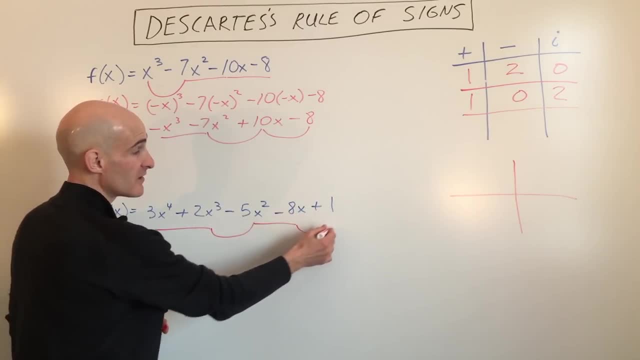 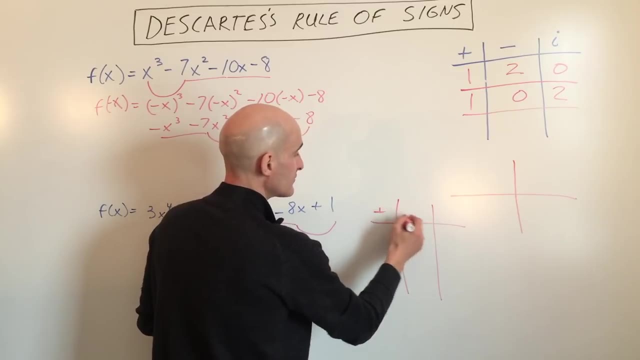 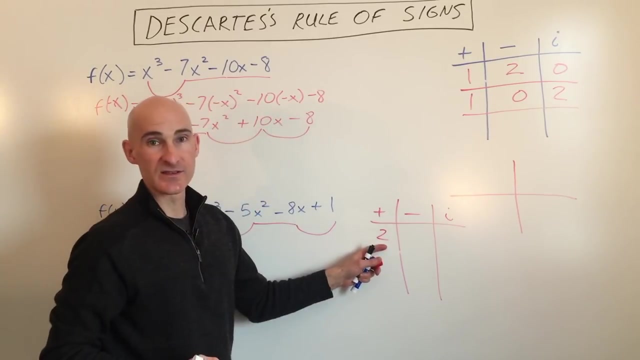 negative to negative doesn't change negative to positive. that's another one. So what we have here is let's make another one of our charts- positive, negative- imaginary. We're going to have a maximum of two positive Zeros. If we substitute in negative x we're going to get okay. so f of negative x we're going to. 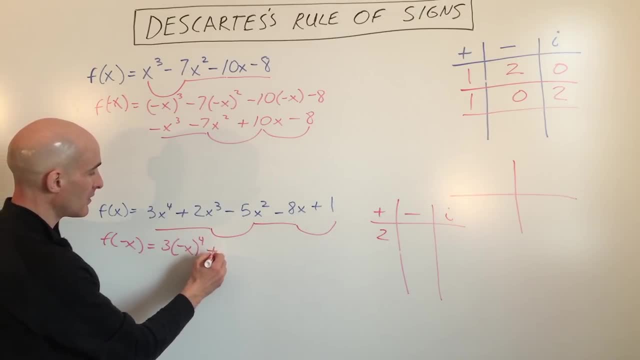 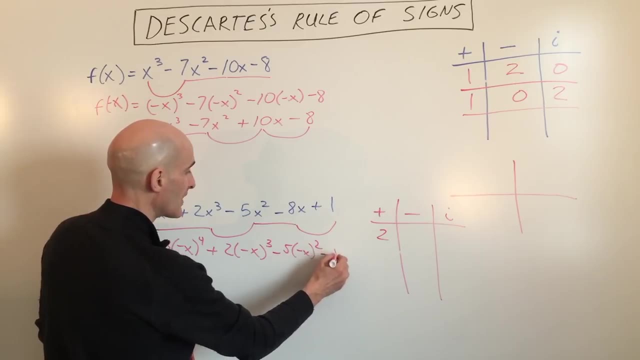 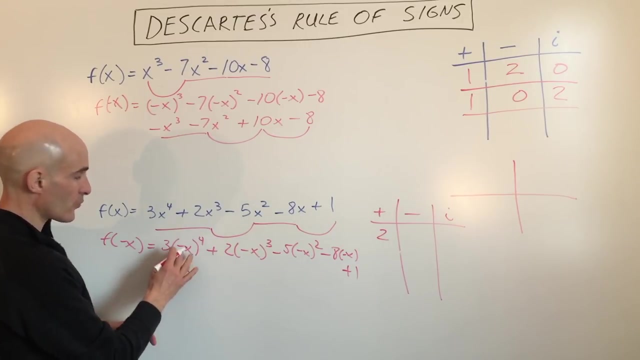 get three times negative x to the fourth, plus two times negative x cubed. minus five times negative x squared. minus eight times negative x plus one. Okay, so here, if we simplify, we get positive three x to the fourth, because a negative to an even power is positive, We're going to get minus two x cubed. 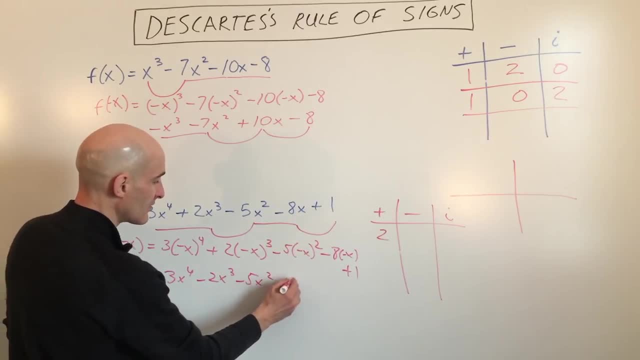 we're going to get minus five x squared. we're going to get positive eight x and plus one. So now let's count the number of sign changes. We have positive to negative. that's one. negative to negative. that doesn't change. negative to positive, that's two. positive to positive, that doesn't. 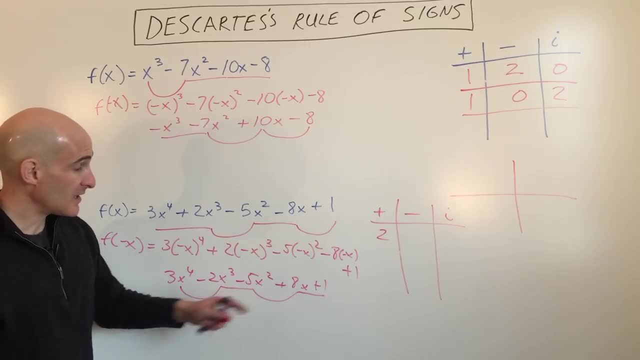 change. So we have a maximum of two negative zeros. Okay, so these are the maximums, and if we add across two plus two plus zero gives us four, and the maximum number of zeros you can have is whatever the highest degree of the polynomial is. So if we add across two plus two plus zero, 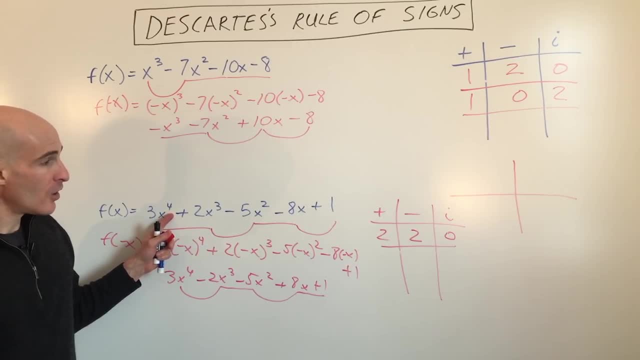 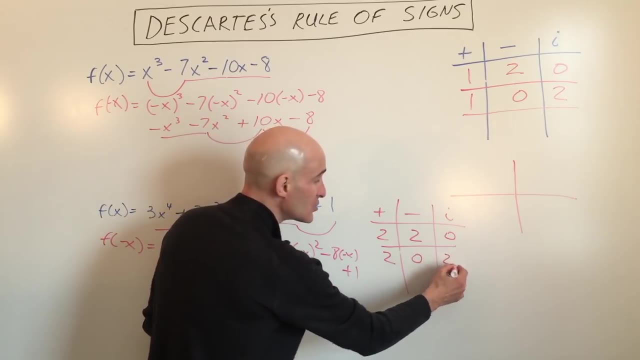 the highest degree of the polynomial is, which in this case is four. okay, so let's look at some other possibilities. we could have two positive, zero negative and two imaginary. notice how this went down by two and this increased by two, the imaginary zeros. or we could have 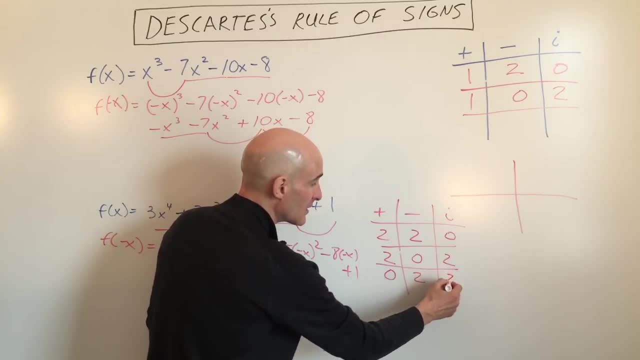 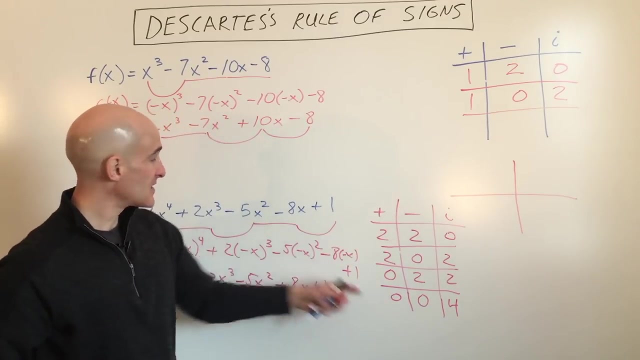 zero positive, two negative and two imaginary. again notice these add up to four as you add across, or we could have zero positive, zero negative and four complex or imaginary roots. so these are the possibilities for this polynomial, okay, this function, and this didn't really help us a whole lot because in this example, 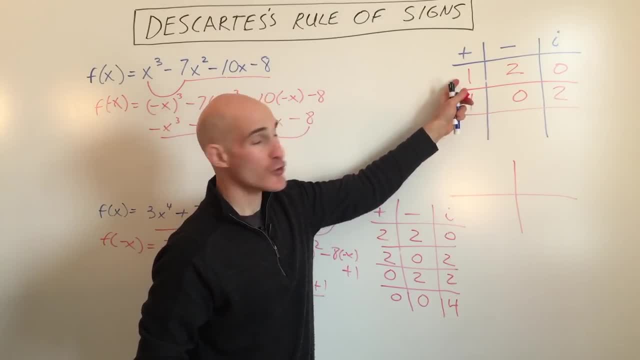 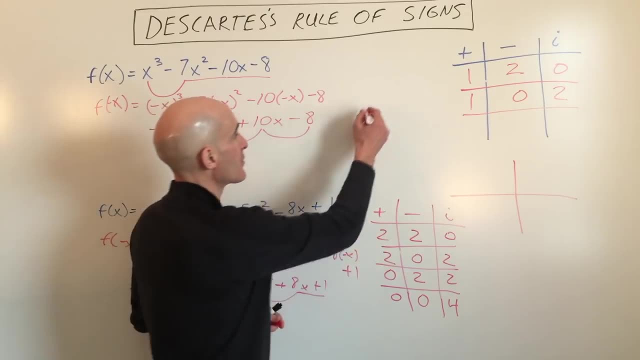 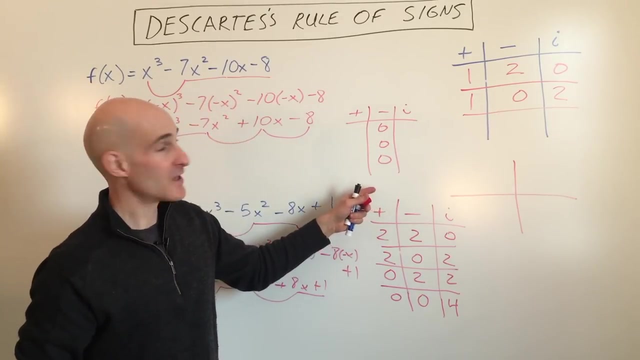 here. we knew that we're going to have at least one positive root, so we could go and try and find that one here. though you know, you'll get sometimes like the scenario where like say, for example, you'll have positive, negative, imaginary you'll have zero negative roots. so you say, well, let me just focus on finding the positive ones, or vice. 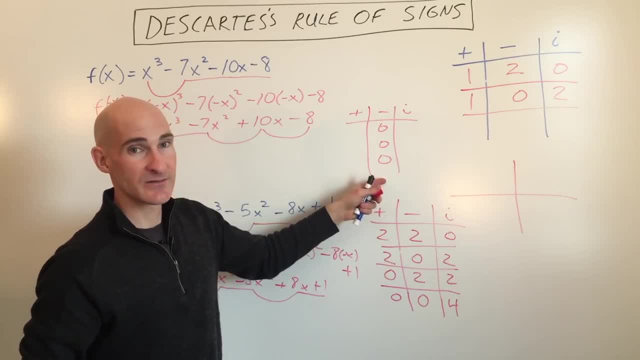 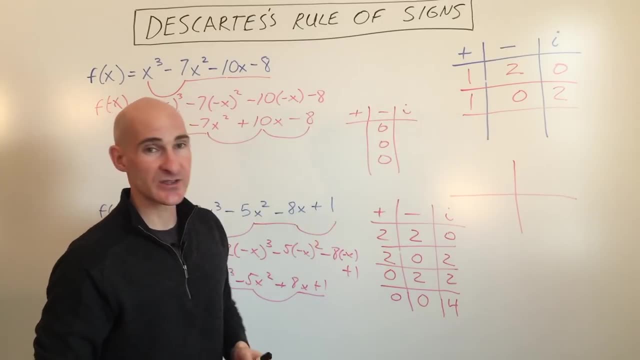 versa. they might be zero, positive and some number of negative ones, and then you can just focus on finding, you know, one of one or the other, depending on what the table does and shows you. so these have been some examples here of how to use Descartes rule of science. 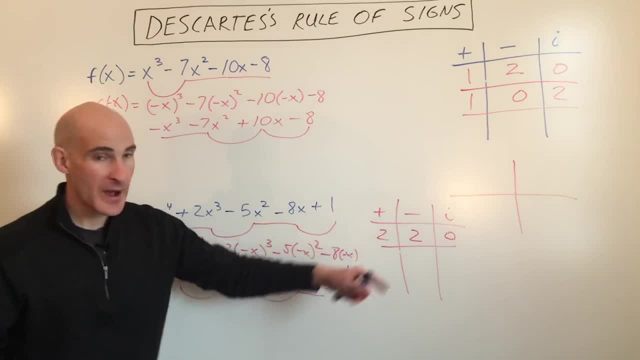 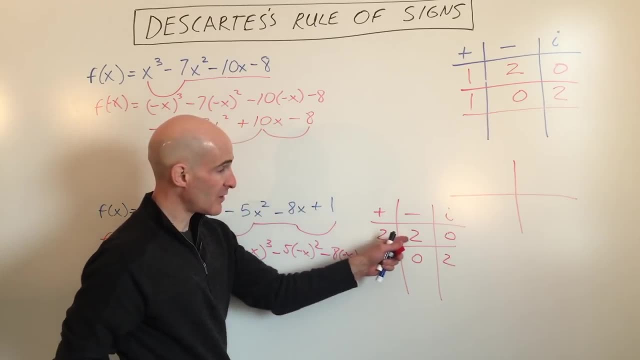 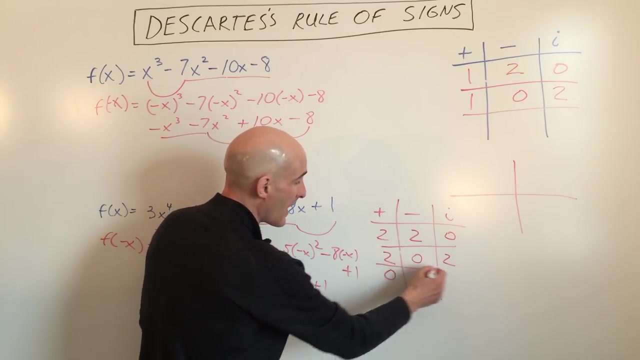 we get four. Okay, so let's look at some other possibilities. We could have two positive, zero negative and two imaginary. Notice how this went down by two and this increased by two, the imaginary zeros. Or we could have zero positive, two negative and two imaginary- Again notice. 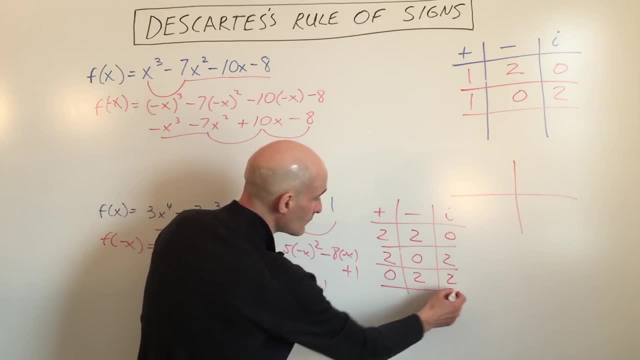 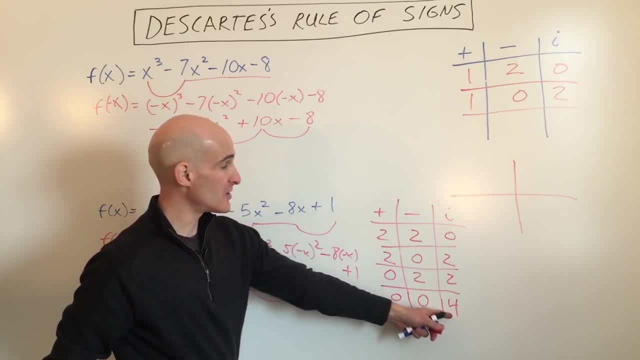 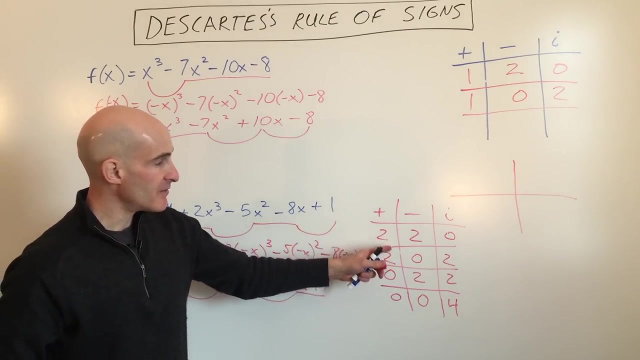 these add up to four as you add across. Or we could have zero positive, zero negative and four complex or imaginary roots. So these are the possibilities for this polynomial, okay, this function. And this didn't really help us a whole lot because in this example here, we knew that 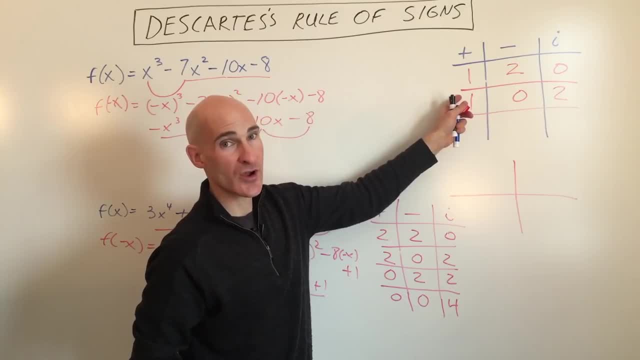 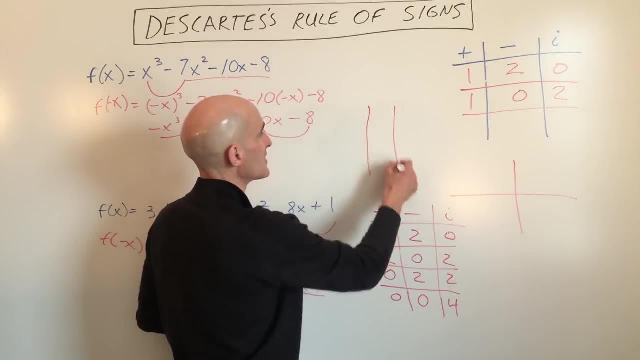 we're going to have at least one positive root, So we could go and try and find that one Here, though you know you'll get sometimes like the scenario where, like say, for example, you'll have positive, negative, imaginary and you'll have zero. 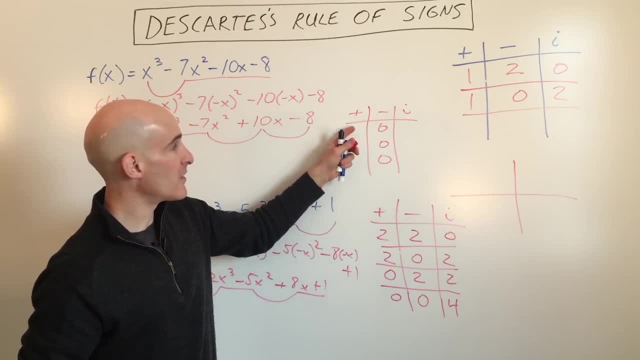 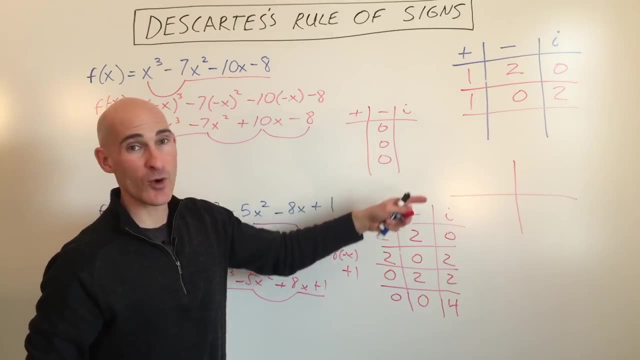 negative roots. So we're going to have zero negative roots. So we're going to have zero roots. So you say, well, let me just focus on finding the positive ones, or vice versa, They might be zero positive and some number of negative ones, And then you can just focus on finding. 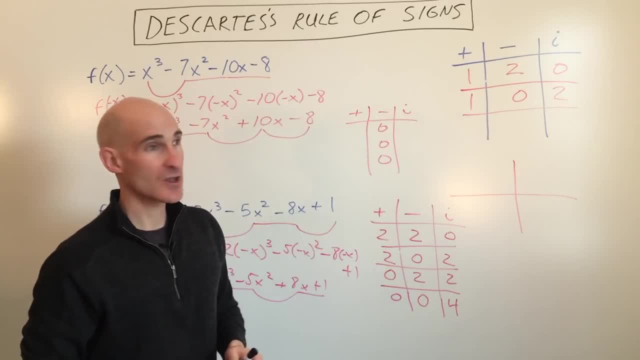 you know one or the other, depending on what the table does and shows you. So these have been some examples here of how to use Descartes' rule of science to narrow down the number of you know choices that you're going to use when you do your synthetic division. So like just to show you just. 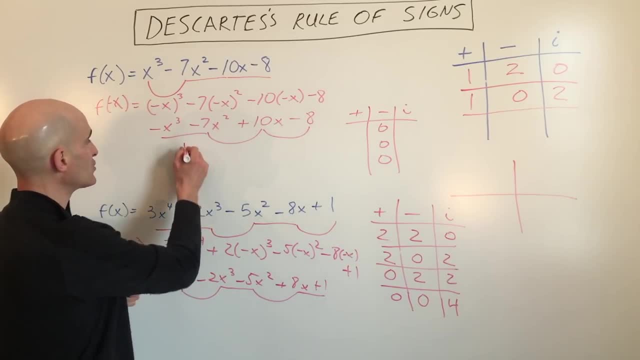 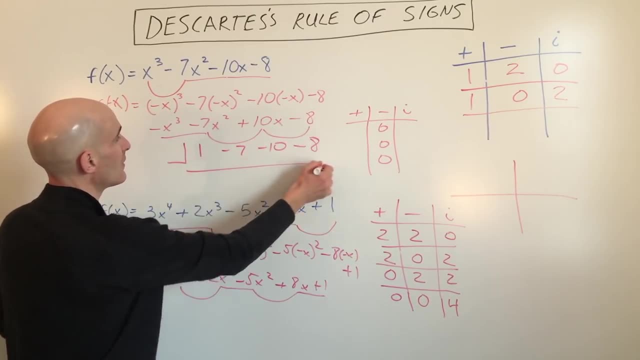 a little bit more about this one here. If I was doing this, I would be doing this, I would be doing synthetic division. Okay, I've got 1, negative 7,, negative 10, and negative 8. And since I 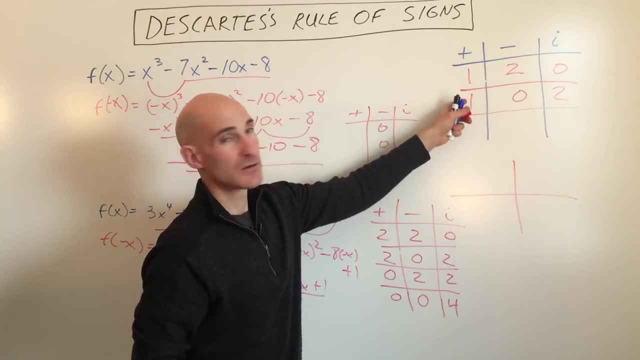 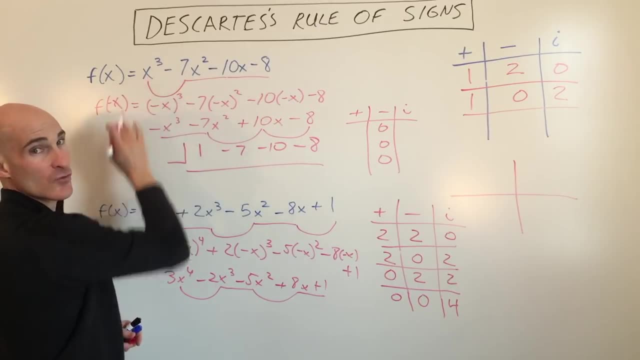 found out, there was at least one positive zero. let me just try, for example, p over q. Okay, so all the factors of 8 over all the factors of 1.. So I know that 1 might be a possible root, So let's. 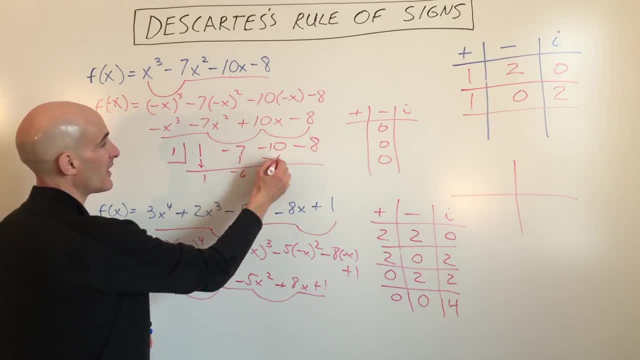 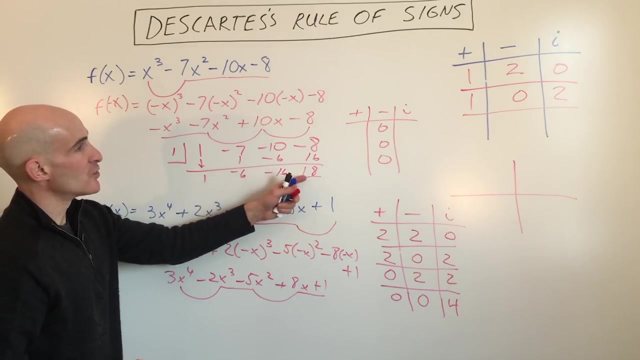 do the synthetic division Multiply, add. Make sure to just write 1, negative 7, negative 10, negative 8.. So that's going to give you negative 16.. That's going to give you 16.. That's 8.. So that's not a zero, So you would just continue. 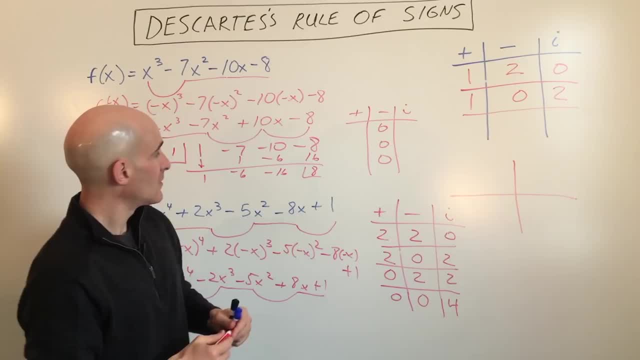 on testing the possible rational roots to see, but we know that there's at least one positive one. So this has been how to use Descartes' rule of science. I'll see you in the next video. 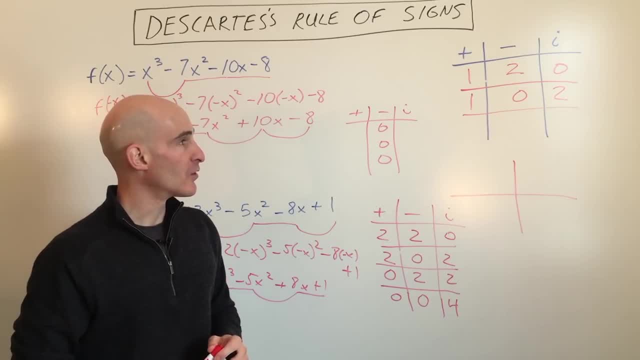 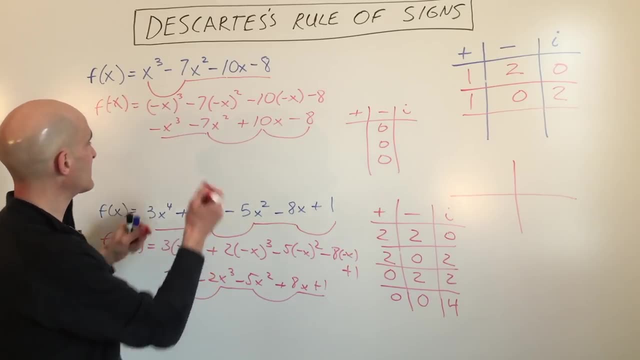 to to narrow down the number of, you know, choices that you're going to use when you do your synthetic division. so like just to show you just a little bit more about this one here. if I was doing synthetic division, okay, I've got one negative, seven negative. 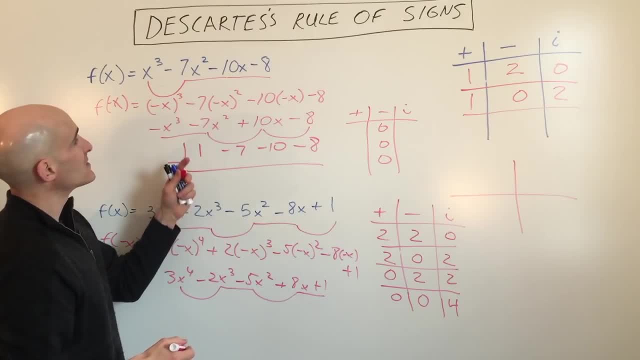 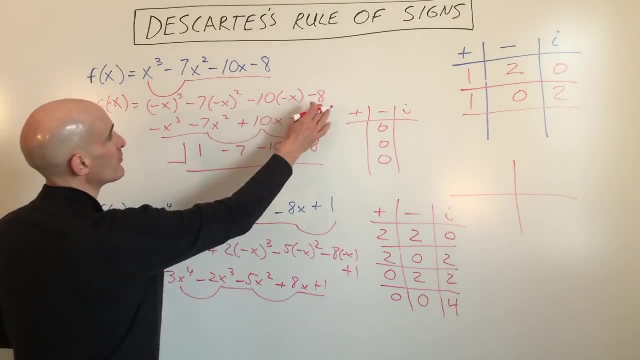 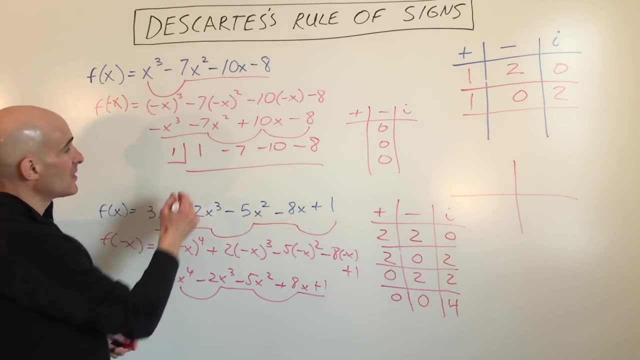 ten and negative eight. and since I found out there was at least one positive zero, let me just try, for example: p over q. okay, so all the factors of eight over all the factors of one. so I know that one might be a possible root. so let's do the synthetic division multiply. 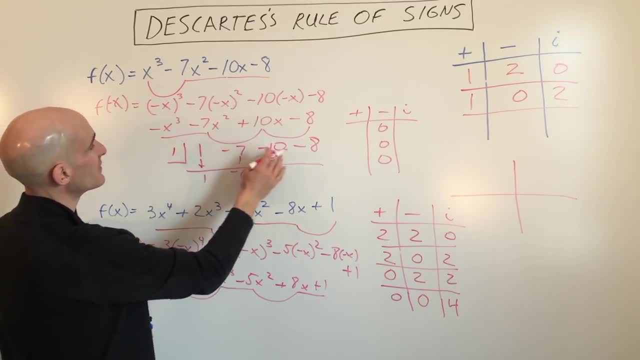 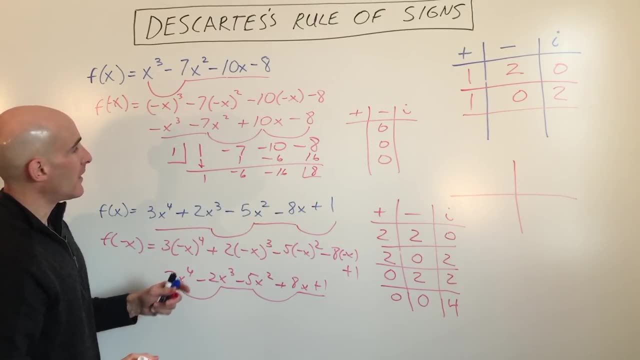 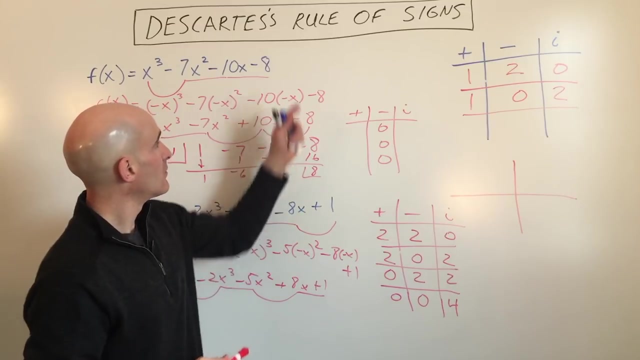 that, make sure, just write one negative, seven negative ten negative eight. so that's going to give you negative sixteen, that's going to give you sixteen, that's eight. so that's not a zero. so you would just continue on testing the possible rational roots to see. but we